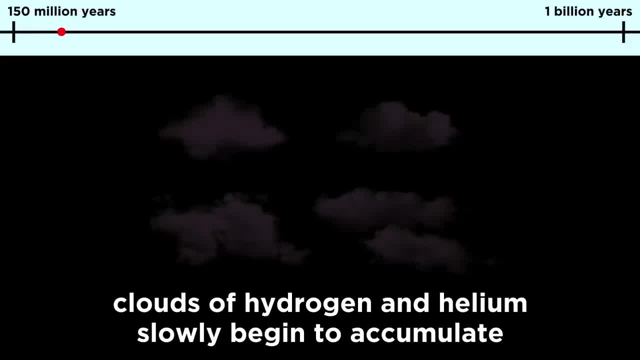 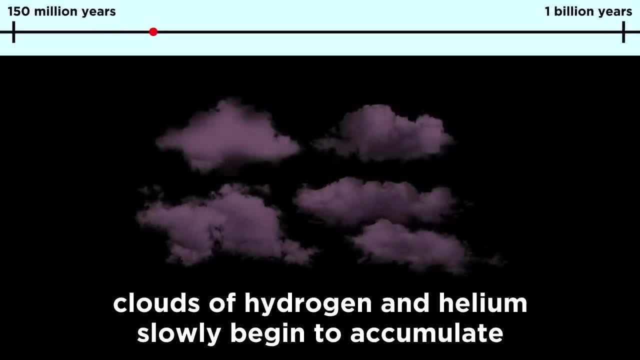 So from around 150 million years to about a billion years after the Big Bang, all of this hydrogen and helium slowly began to collect into regions of higher density. Given the random distribution of matter, some regions became very dense quite early in this era, while others took a lot longer. but let's zoom in on one of these dense patches of gas. 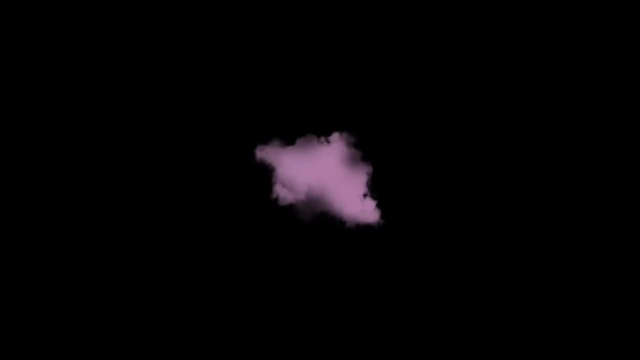 to get a closer look. We know from study and research that gas is a very dense substance. We know from study and research that gas is a very dense substance. We know from studying gases in chemistry that particles within a sample of gas will exert a certain pressure or outward force. 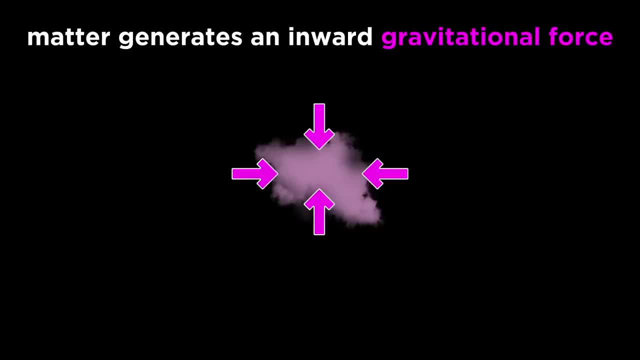 But we just said that all matter exerts gravity, which will manifest as an inward force towards the center of a large gas cloud. By large gas cloud. we aren't talking about the clouds we see in the sky. We are talking about clouds at least a light year across and often much larger. so this 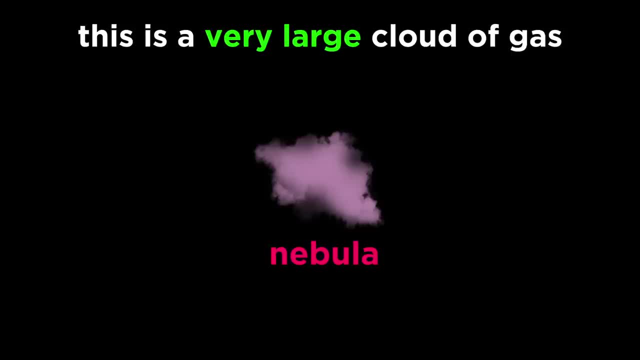 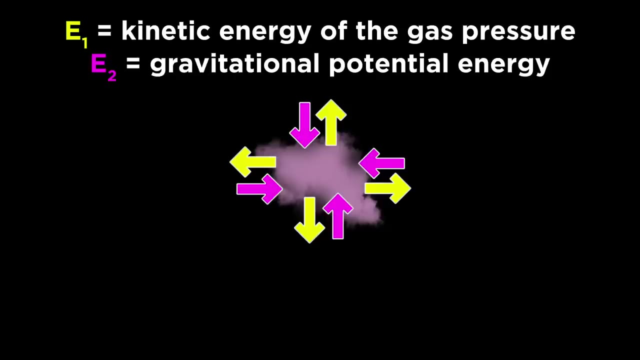 is quite a lot of matter involved. A cloud like this, also called a nebula, will remain in equilibrium if the kinetic energy of the gas pressure or the force pushing out is precisely in balance with the gravitational potential energy or the force pushing, in a situation called hydrostatic equilibrium. 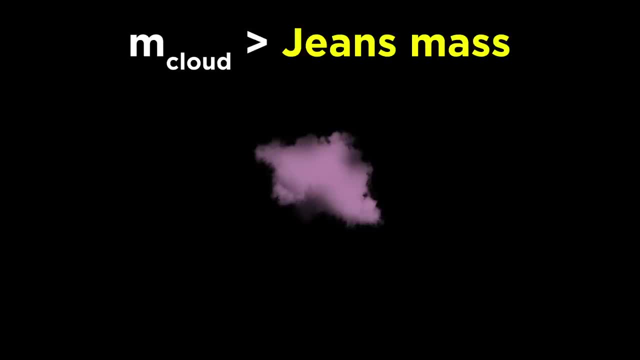 But if a cloud is massive enough above a threshold called the Jeans mass, which is usually at least a few thousand times more massive than our sun, gravity will increase easily. win the shoving contest and the minimal kinetic energy from the cold gas pushing out. 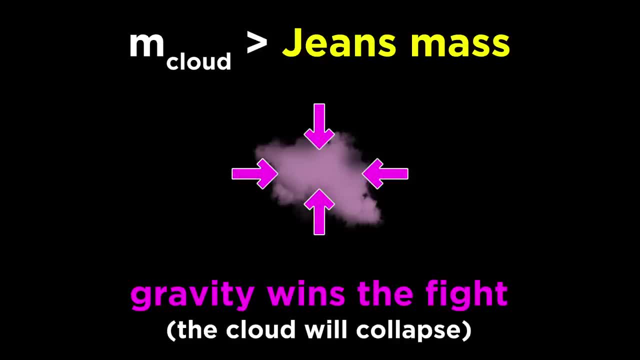 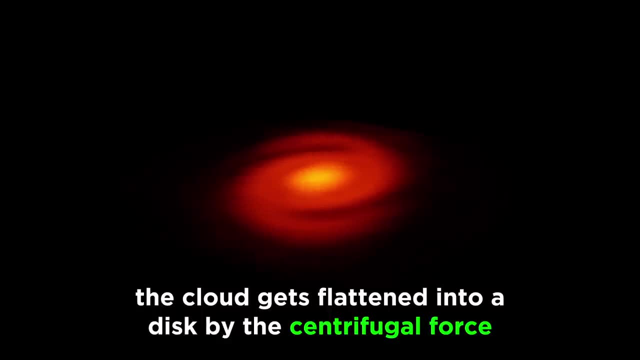 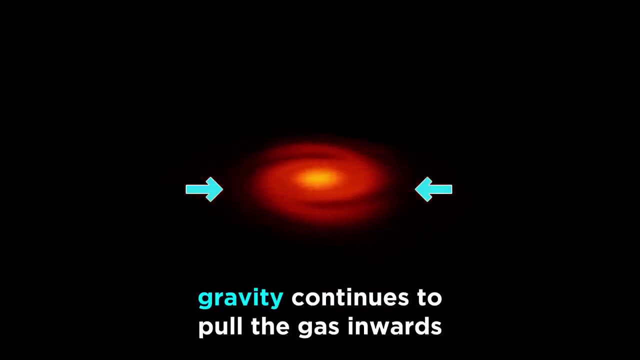 will not be enough to prevent gravitational collapse. Any net rotation is amplified as the cloud gets flattened into a disk by the centrifugal force, like a pizza chef spinning dough in the air, with gravity pulling matter towards the center of the disk. The precise physics involved does get rather complicated. but to make a long story short, 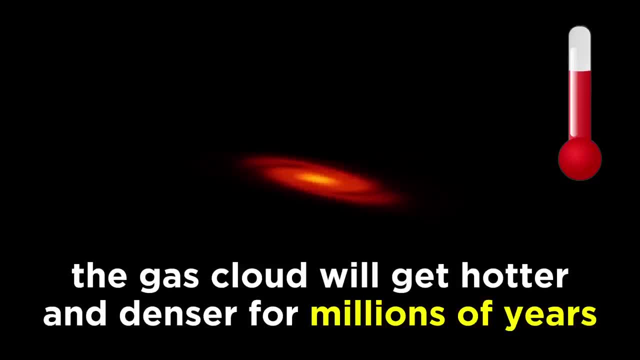 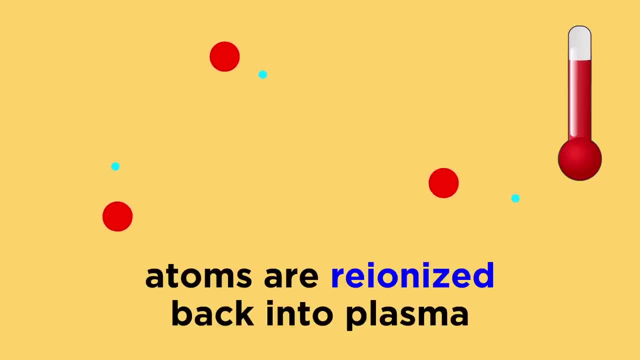 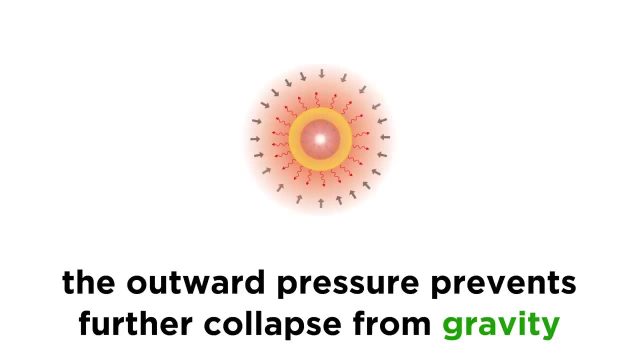 it's much harder still as the collapsing continues over millions of years until the atoms are re-ionized back into plasma, with temperatures getting too hot for neutral atoms to exist. Eventually, the inner region of gas is so hot that the outward pressure supports the. 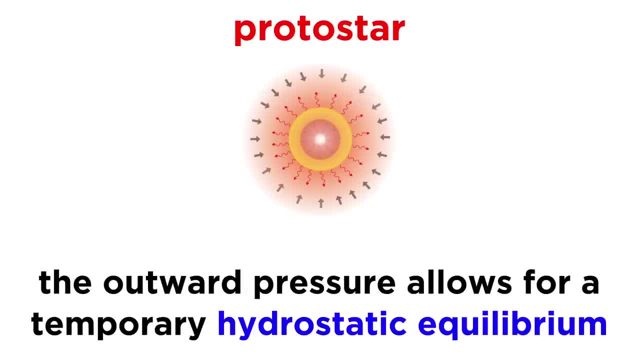 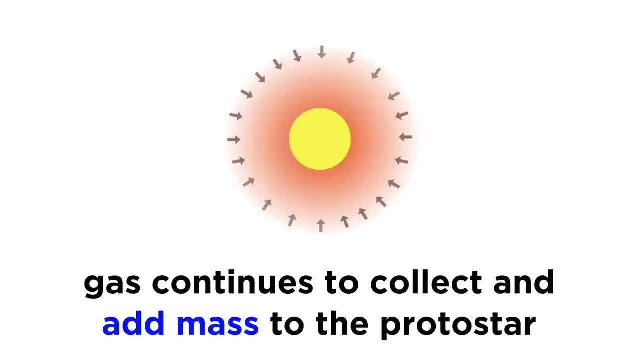 gas against further collapse, and we call this a protostar, an object that is in a temporary hydrostatic equilibrium. More material from surrounding gas continues to collect on the protostar, increasing the gravitational potential energy With sufficient additional mass. collapse then continues, with the inward pressure becoming 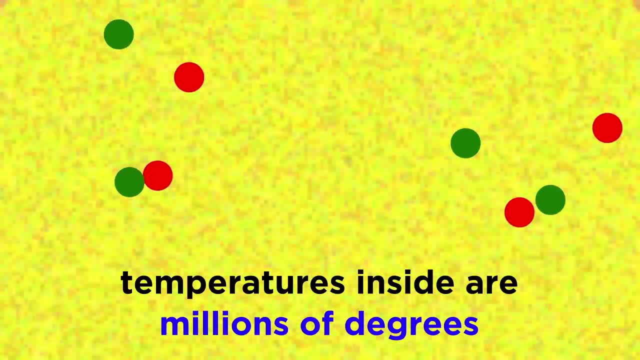 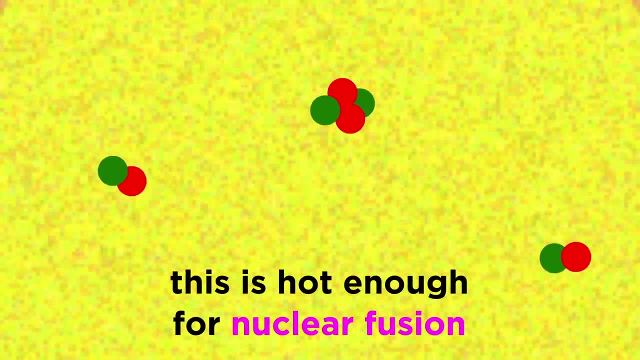 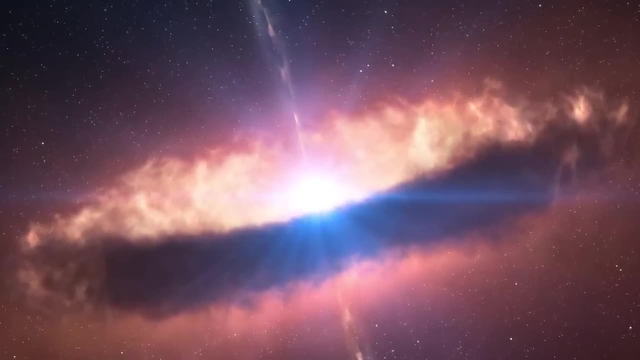 so great that it causes temperatures to rise to millions of degrees until things are hot enough for nuclear fusion to occur, along with the tremendous energy that fusion generates, And with that a star is born. While this depiction was certainly oversimplified for our purposes, it will suffice to imagine: 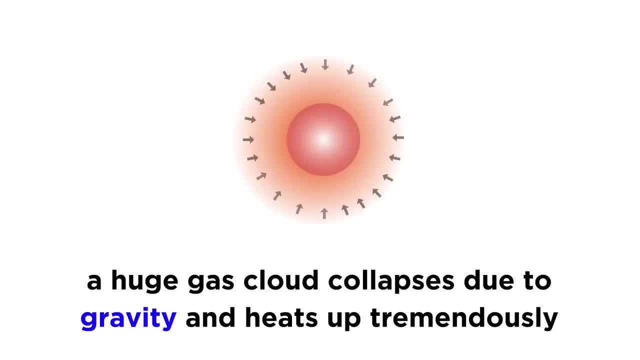 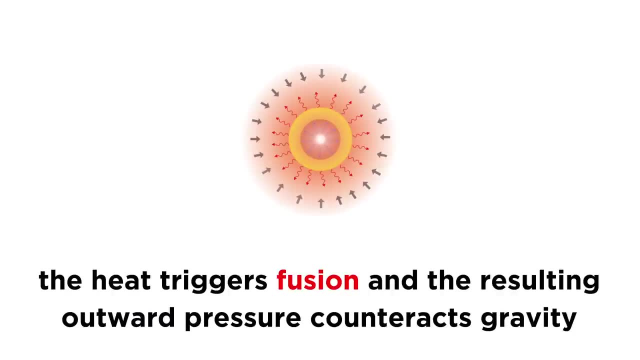 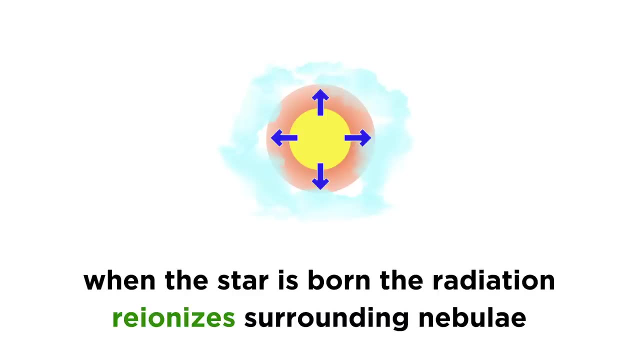 a star as a gigantic gas cloud that collapsed on itself with such tremendous gravitational force that it heated up until it became a spherical furnace of plasma, a hot soup of nucleons and electrons. whizzing around. The formation of this star results in tremendous radiation, which will trigger re-ionization. 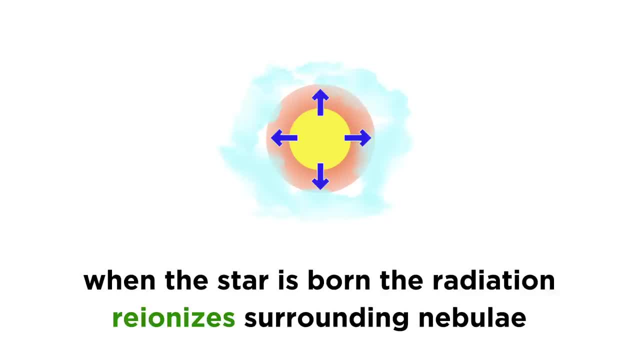 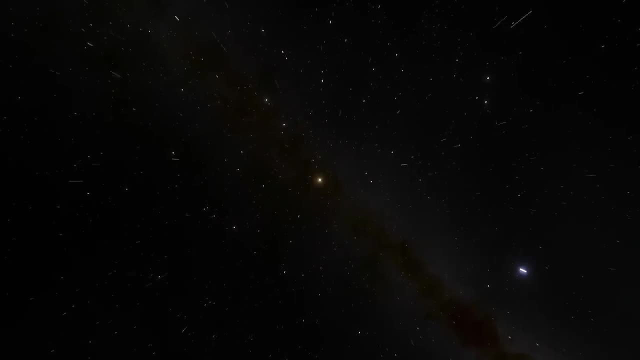 in surrounding nebula, Stripping these gas particles of their electrons. This radiation can also push regions of gas around to collide with others, in turn promoting more star formation. The precise nature of each star depends largely on its mass, and later we will talk about. 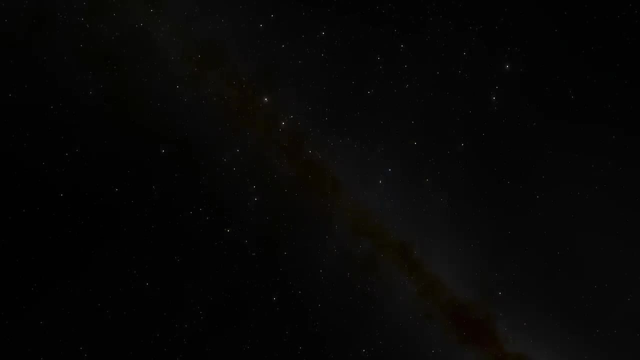 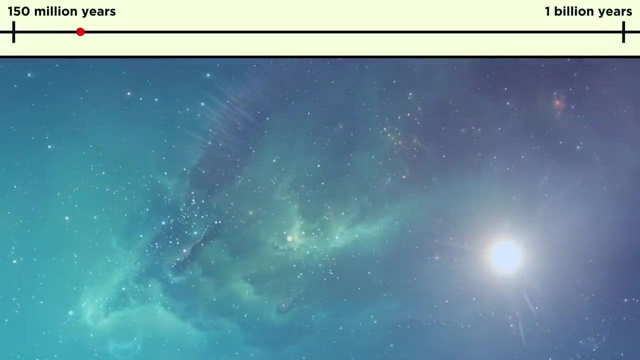 all different kinds of stars, how they form and how they die. But for now, just imagine that during this period, stars are forming all over the universe slowly For hundreds of millions of years, lighting up the once pitch-black cosmos and bringing 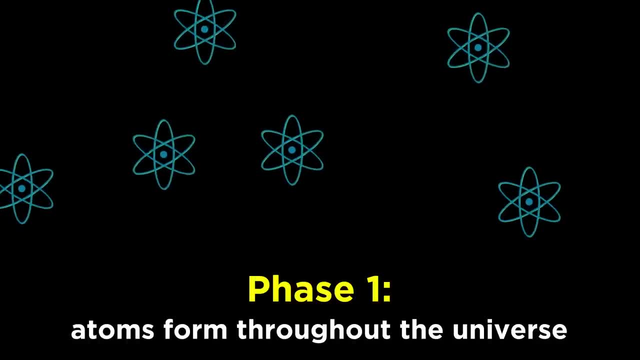 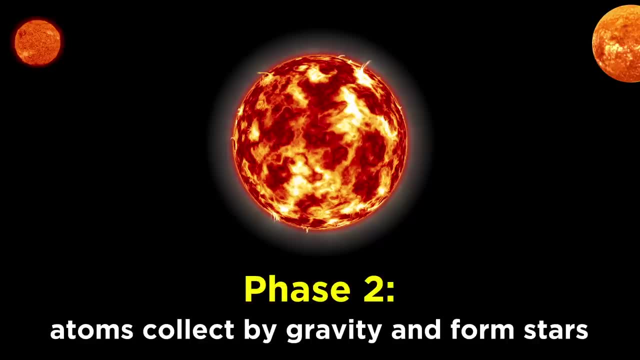 the dark ages to an end. So we've gone from tiny atoms scattered around the universe to huge stars burning hydrogen fuel and glowing like fireflies. What happened next? Well, the key factor will continue to be gravity, as will be the case throughout our astronomical 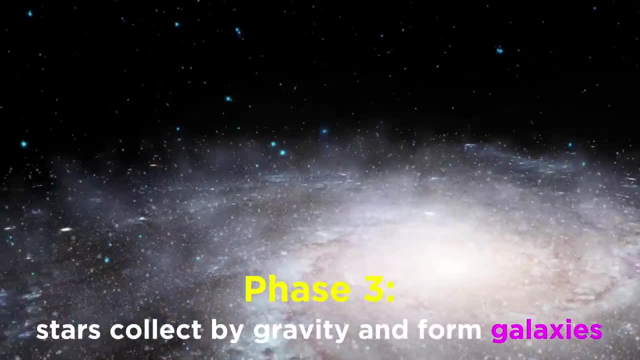